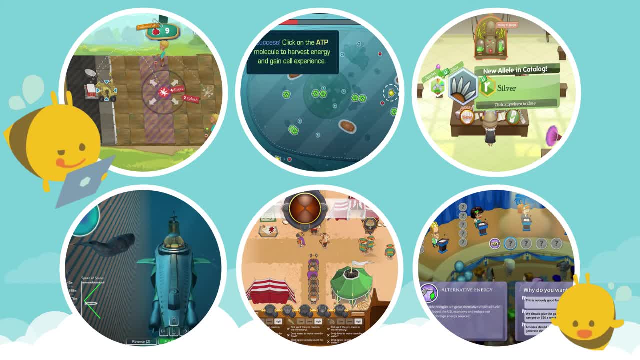 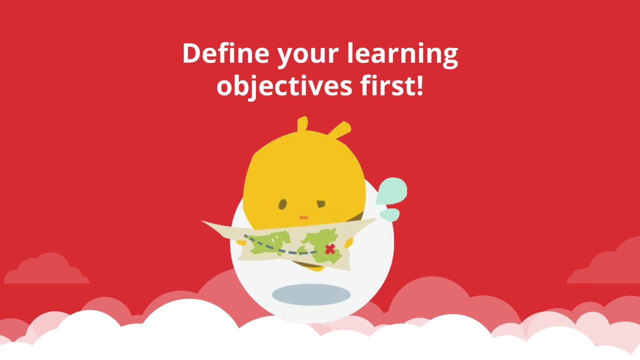 discoveries and make entertaining mistakes along the way. So let's sort of talk about how Filament approaches making these games so that they turn out not as piles of junk. The first step for all of our games, all of our learning games, start with the very the very same first thing, and 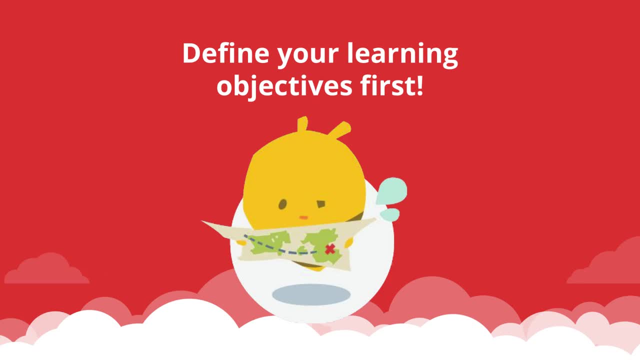 that's defining your learning objectives. That may seem sort of obvious. right, You're going to make a learning game. you should make a learning game. you should make a learning game. you should know what you intend someone to learn. But it's very important to get it documented right away: get. 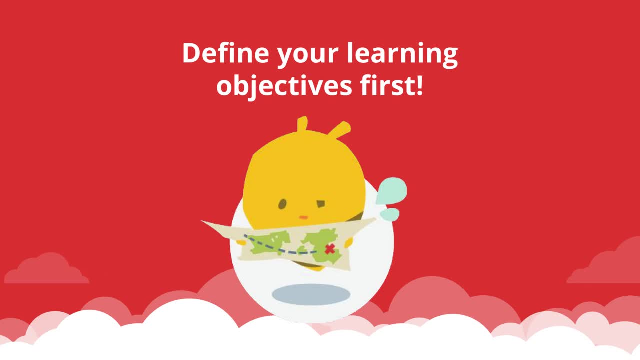 everyone, to get a consensus, understand what it is. someone should know, once they're done playing the game, Things that can go wrong. if you don't do that is you may have different levels of understanding of how deep something should be understood, or it's maybe the topic for the wrong. 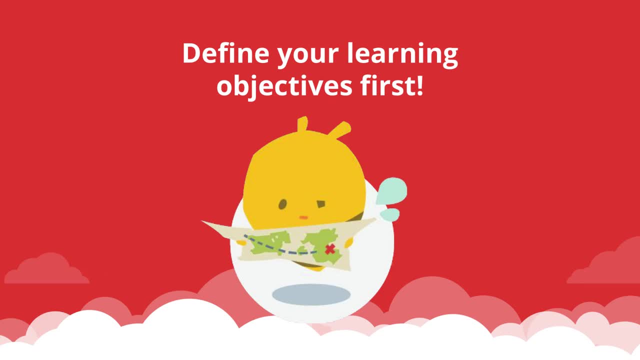 audience, or even, you know, in some cases there's there's disagreements about what that thing even is. So it's very important to have a clear understanding of what that thing is and to be able to understand what it is that you're trying to learn. And that's the first step, And then the last step is: 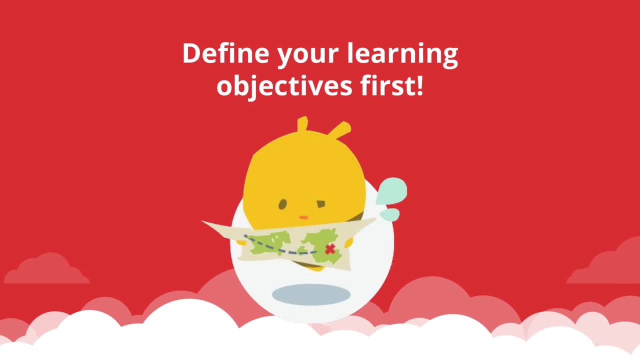 to define your learning objectives And that's where you're going to have to go from one way to the other. So deciding on a source and a pedagogy and a practice, making sure all those things are poured into your learning objectives so they're nice and clean and clear, is is absolutely critical. 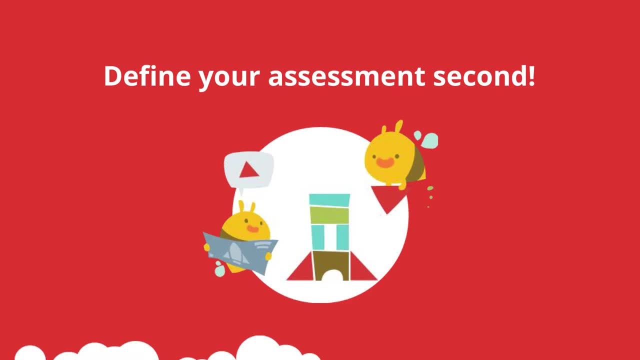 After you've defined your learning objectives, there's still one more step before you get to like some players. not only do you have to declare what you expect that impact to be, but also how are you going to know that it worked. I know that sometimes the word assessment sounds like it can. 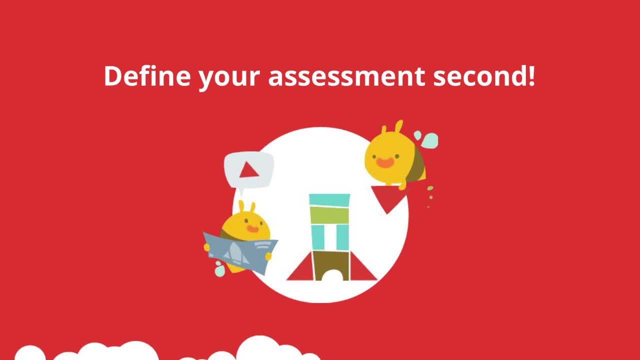 be a negative thing, But we're really just talking about what do you think is a fair way to decide that someone has been positively affected by what you've made? So this doesn't need to mean that they taking a a bubble multiple choice test or answering some true falses. you know you can set. 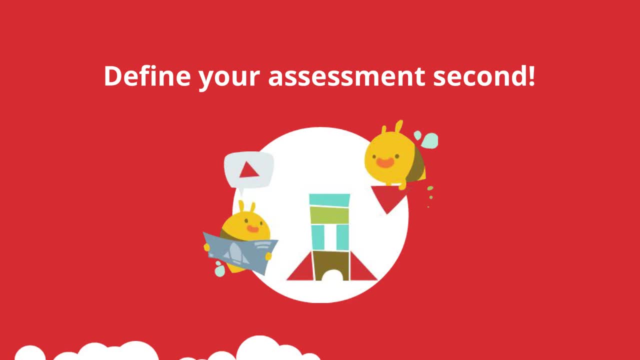 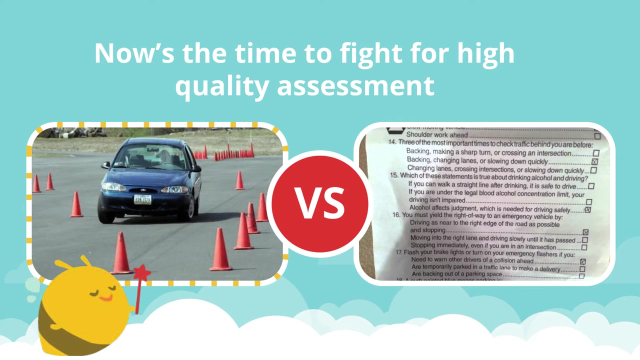 assessments at any level of evaluation that you want, But it's good to be open and honest about how you expect to assess your learner at the end, so that that way you know that you're not going astray when you're designing the game mechanics. I think a simple and great example for this is the American driver's license system. 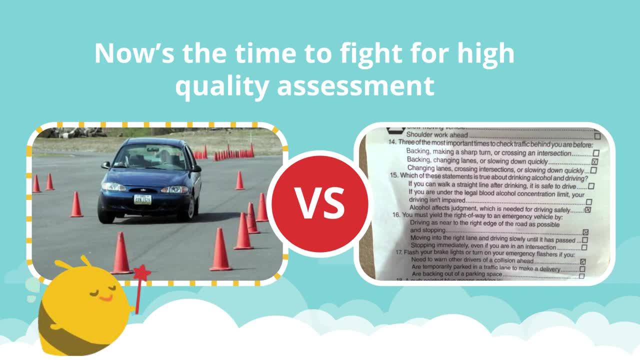 In order to get a driver's license, it's considered fairly obvious that you definitely need to get behind the wheel of a car. someone should watch you drive that car and decide whether or not you're going to wind up murdering people with that car. 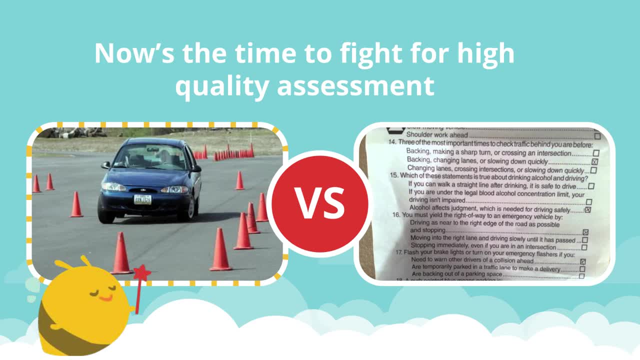 007, And if they think that you're going to wind up murdering people, you don't get your license yet. 008. That seems very clear, right? You want that. you want to know that people have had a live, high quality assessment of their driving ability And I'm sure many people even feel like that bar. 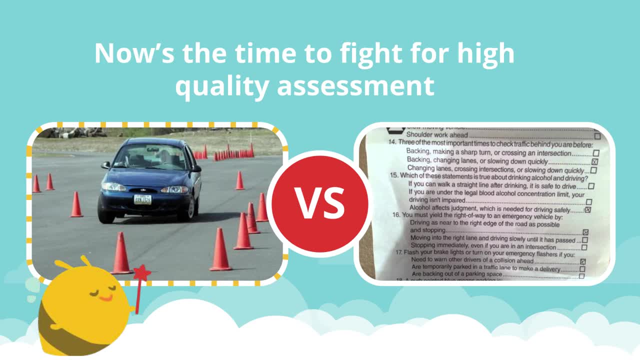 could be raised even higher. it would be a sort of- even you know a scary universe if we just gave people a written test and said: Hey, take these 20 questions And tell us, tell us whether or not you can drive via this people's license system. 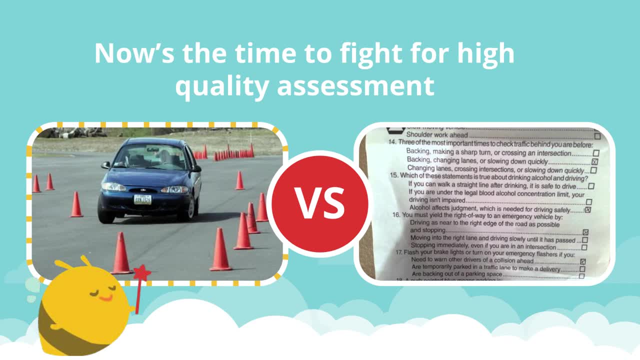 009, And that sounds crazy, right, And it is. you know, perhaps a piece of commentary that there's so many other really important things that we decide can be sorted out with pieces of paper. But this is sort of the time during your early design stages to say, Hey, what's the, what's the best most? 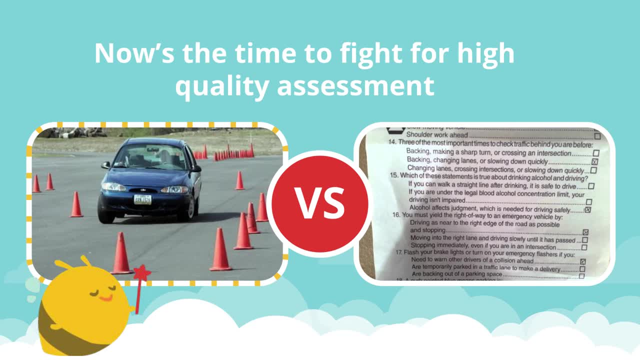 powerful way to assess whether or not we know a thing when we're done playing this game. And let's aim for that, Let's, aim for that, Let's. let's go for that depth Right. That type of depth will actually make the rest of your game design easier. 009. 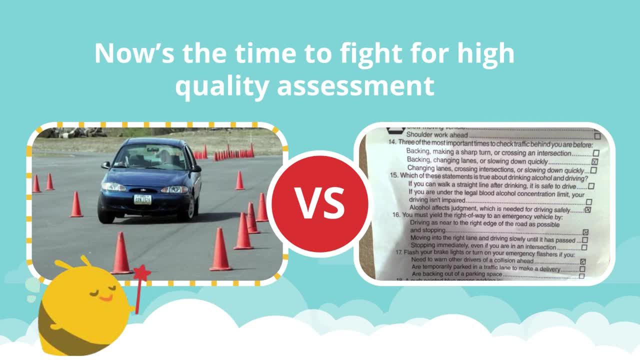 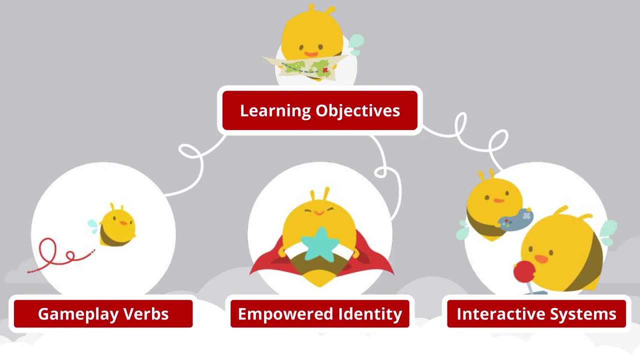 It is hard to make what you would call a great learning game if your expected outcome on the other side is to take a paper driven assessment. So we've got our handy dandy learning objectives all set And we've got our assessments, and those are dutifully documented. 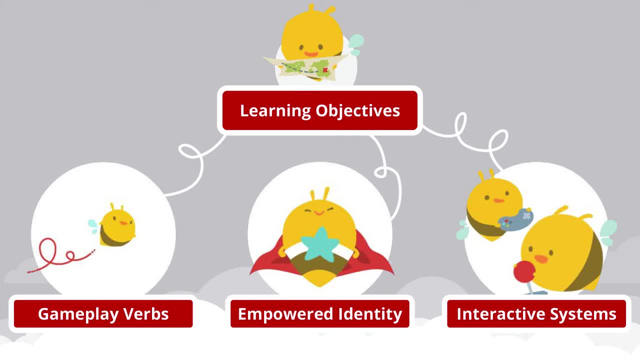 Now is the time to start turning those objectives into gameplay mechanics. So when I say mechanics, I mean the rules that govern the interactions inside the game, So the things that sort of drive the game to make it a game. Filament uses sort of three core strategies for migrating. 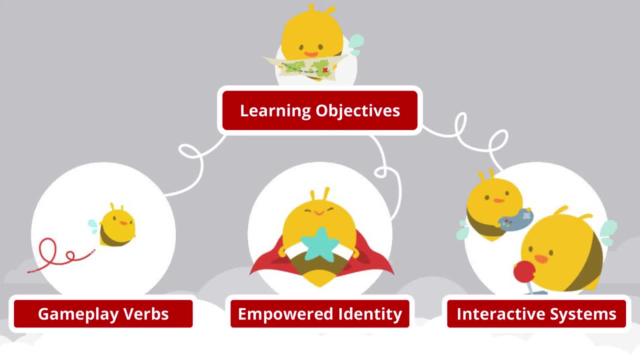 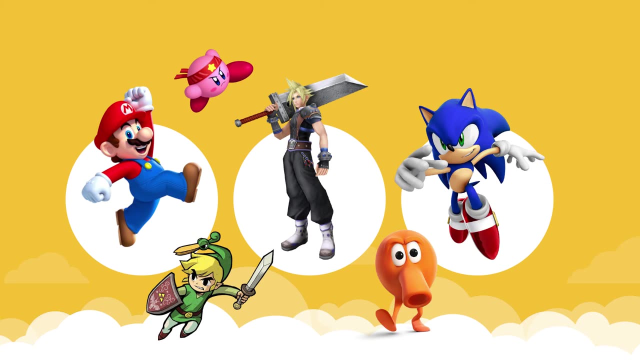 learning objectives into gameplay ideas, into gameplay mechanics, And I'll go into a little bit detail on each of them Very quickly. they are verbs, identity and systems. So the first feature I'm going to talk about is identity Games. do this really cool thing where? 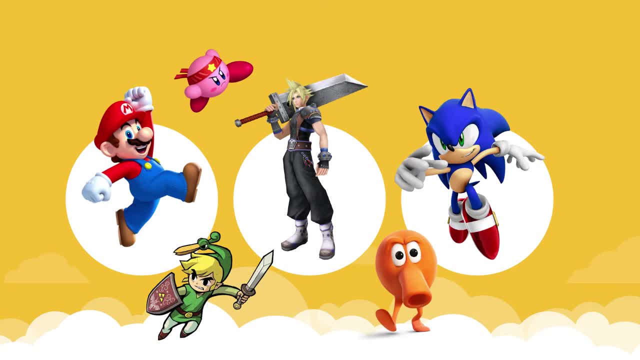 they step into a role, and sometimes that role is a named character like Cloud or Sonic or Qbert, as we can see here, And sometimes that role is a profession. But they ask you to sort of merge yourself with some sort of identity inside the game and players just say, Oh, okay, that sounds. 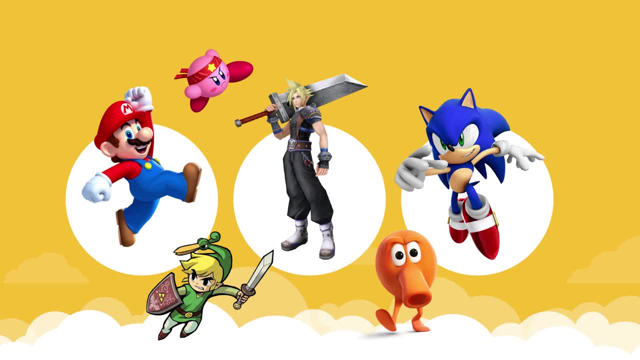 great, now what? And that's really cool and interesting. It's a very unique thing to games 009. I often say that. You know, games are pretty unique in that it's very rare to see other forms of media that work with the player in the second person. 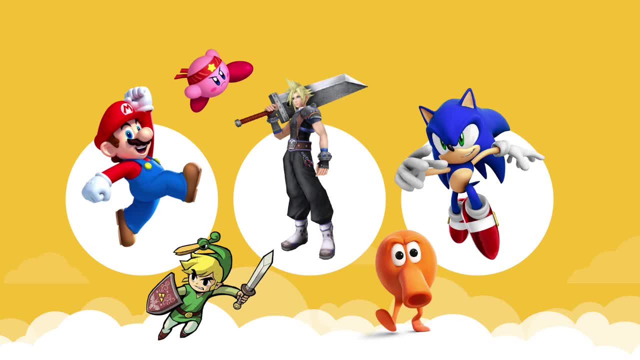 You know games talk to you and you do these things and you have these capabilities, And players reflect on those things then in the first person, even if they are not seeing the game through the eyes of the player in a first-person camera perspective. 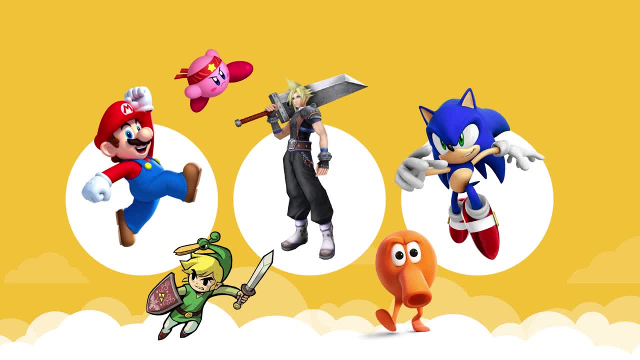 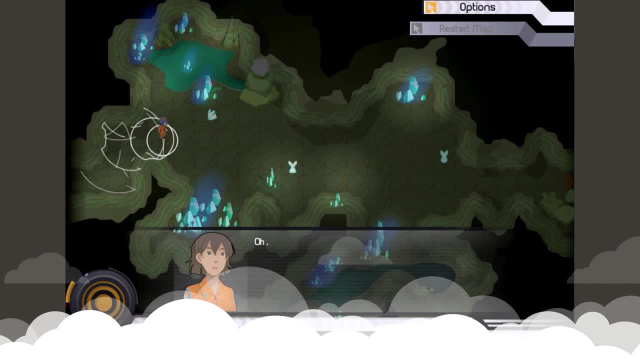 They generally are given an identity and they react inside the game space from that identity. I think a quick example from Filament is we made a game called Prisoner of Echo where you're given an identity of a scientist attempting to escape an underground and yet still in outer space research facility. 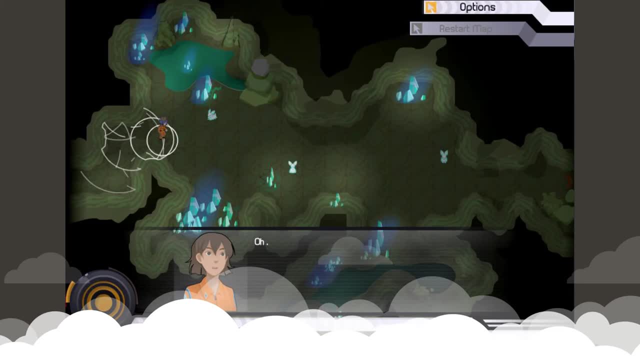 Your entire identity in that game is wrapped up with the ability to understand and control sound, And so we have this blend of your science, You have your scientific goals with your skills, and they all sort of speak to who you are and how you're empowered to do what you're going to do in that game. 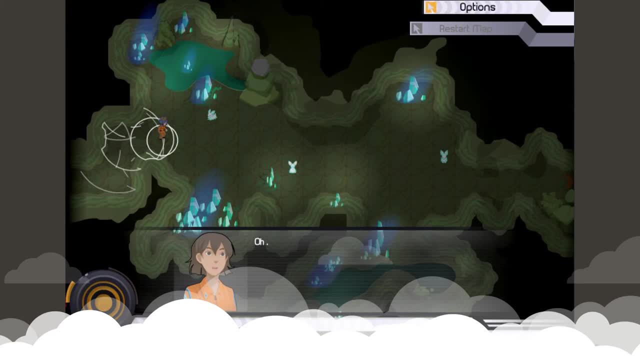 So, if you have learning objectives that focus on how to see the world from a perspective that maybe you're not used to, or how to embody a particular professional practice or a way of thinking or a way of socially interacting, all of those types of learning objectives. 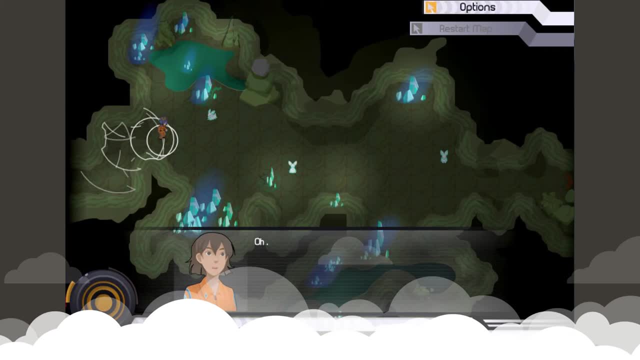 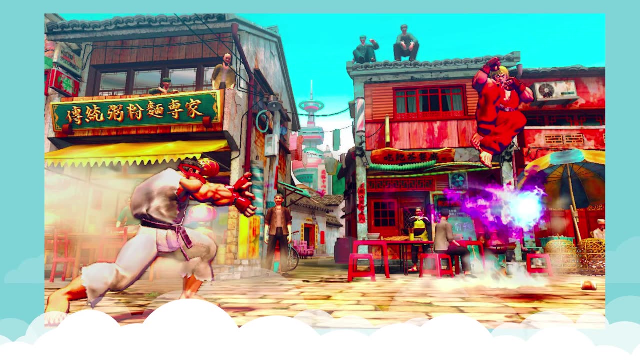 Maybe ripe candidates for using identity to build game mechanics. The next is verbs. I think most people- this may be the first, most obvious facet of what games can do for learning objectives. Games can create things to do and they can create digital metaphors for doing all sorts of things. 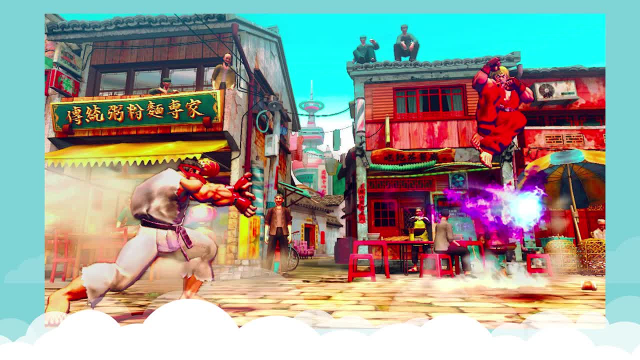 This is obviously a picture of some fighting, which is a thing that games can do. Games are very famous for being good at, but even in the commercial game arena there's lots of games that are about traveling or being a lawyer and lawyering, or cooking, performing surgery. 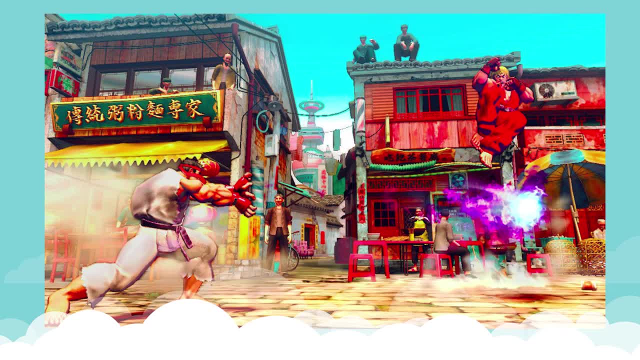 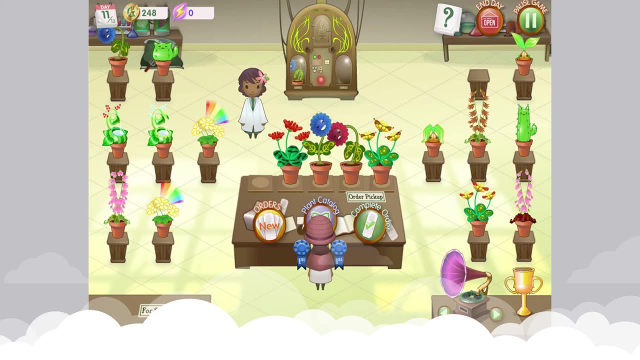 There's a whole wide variety of verbs that go into games and it's a very powerful thing. So a nice example from my filament game is Crazy Plant Shop. Crazy Plant Shop is a game that puts You have customers who come in who require orders of exotic plants and it's up to you to breed those. 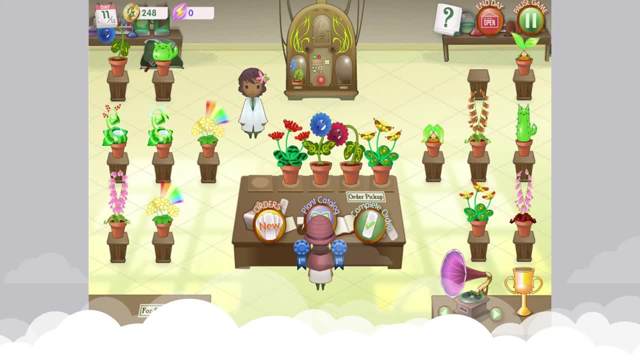 And so breeding as the verb inside this game involves using your science fiction-y machine in the back to lay out the punnett squares of dominant and recessive traits and breed the plant that you want over and over and over, So that core verb. 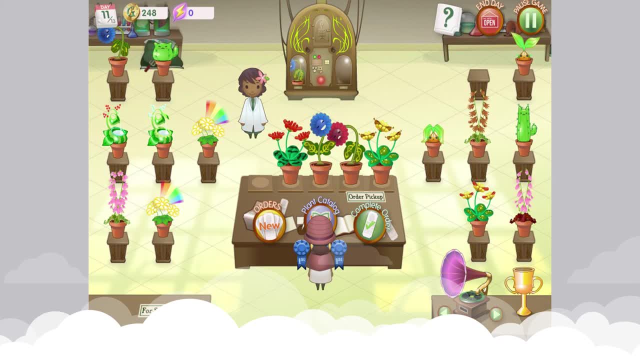 The verb of using the punnett square machine in the back lets you get a ton of great practice on the ins and outs of dominant and recessive traits and the punnett squares that diagram them. So if your learning objectives have some type of action that you'd like the learner to be able to do and you see a clear path to creating a digital version of that verb, then you can do. 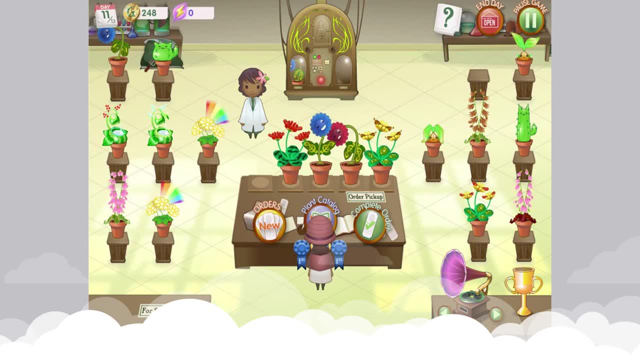 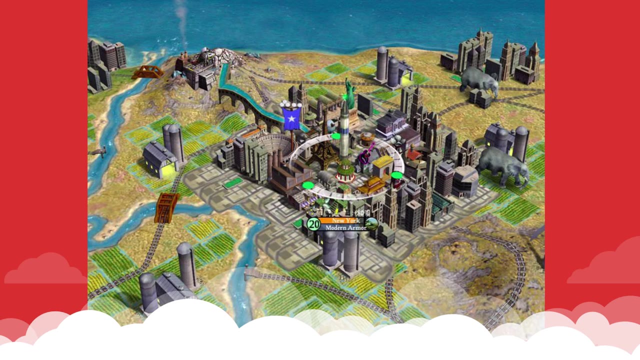 You know Great high-quality wrapper of scaffolding and feedback and empowerment around that verb and build your learning game structure around that with a lot of confidence. The last of our three strategies is systems right. So games are obviously made out of rules and those rules govern how the player interacts inside the space and what does the game's world do in reaction to what the player does. 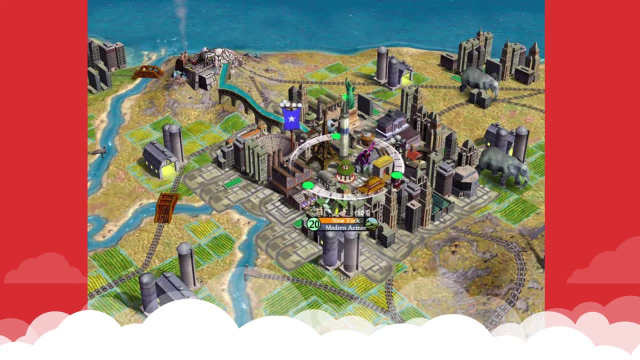 So the fact that games can make living and dynamic sets of rules to create those systems you interact with is one of the really unique and cool facets of game-based learning. So there's lots of classic entertainment games that feature systems thinking as a premier facet of strategy. 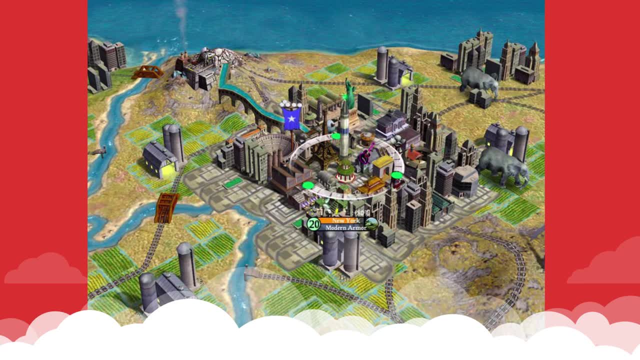 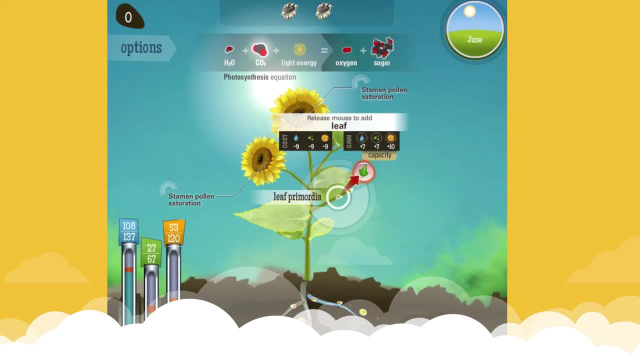 Games like SimCity and Civilization, et cetera, are some of the most obvious examples. Filament has used systems as a premier strategy in games too, So we made a really lovely game called Reach for the Sun, in which you are learning about plant anatomy and plant function. 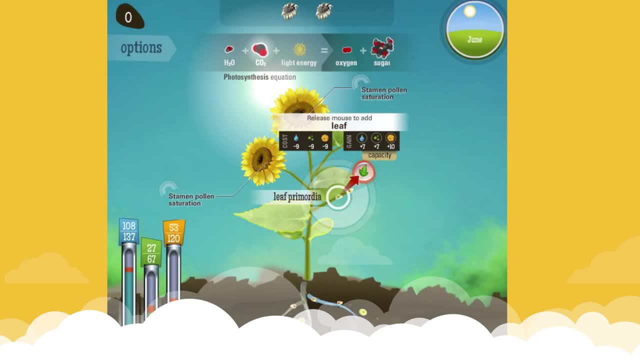 And in that game you interact with a single plant as a system in itself. You decide which pieces of the plant by anatomy that you're going to develop and each of those pieces interacts with your ability to generate. You generate and store resources and you're attempting to manage your resources intelligently over the course of a year to try and flower and fruit before winter comes. 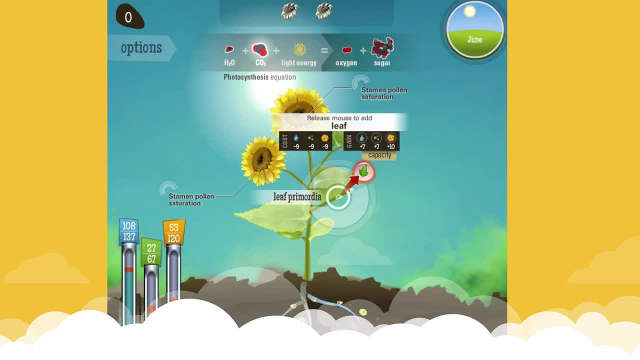 So by using the system with a set of interesting inputs and outputs, we can get you to think about how the parts of a plant work together in a, not just in like a. oh, I can identify all the parts of a plant because I memorized the terms. 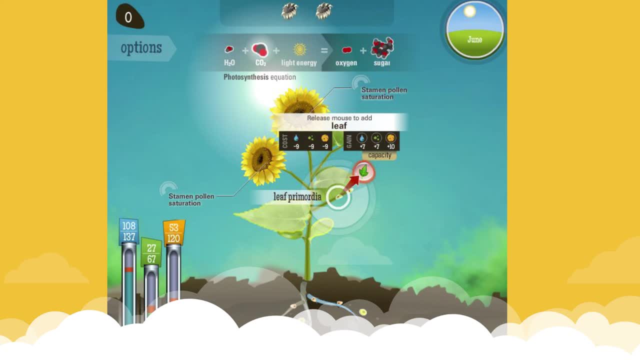 but you actually think of the plant, So you can think of the plants as a set of things that work together to accomplish complicated goals, And that's very powerful. I think systems thinking in games itself is great, because even if you do forget exactly what the parts' names are and the specific terminology, you'll remember the overall puzzle, the overall shape of how those things work. 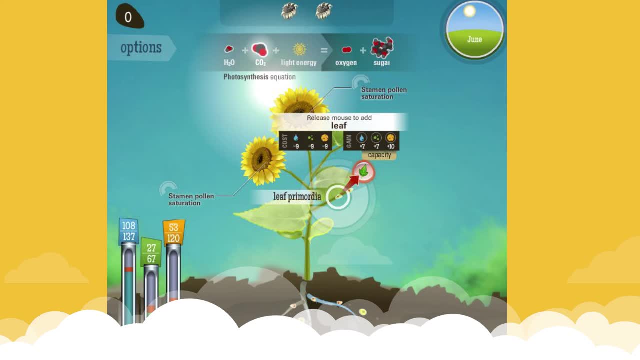 And future work in the classroom or other learning environment. you have sort of a framework to hang more information. you know, because you know what it looks like. Yeah, looks like in motion, with the parts spinning and working with each other. So if you have learning, 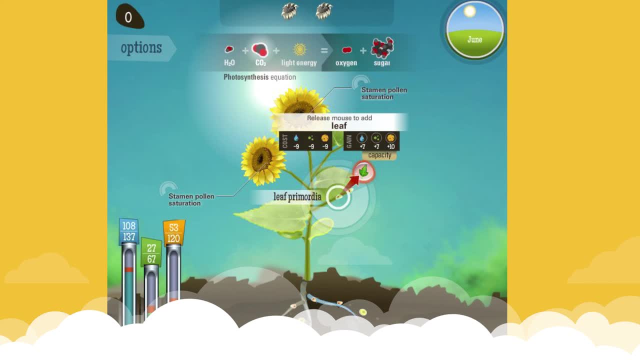 objectives that are about thinking about an ecosystem or a complex interaction of multiple agents. anything where a system is applicable to understanding the objective, you might want to think about turning that system into a set of rules that govern the game and asking the player to interact with them and master them, to be good at it. There is, you know, one thing to keep in: 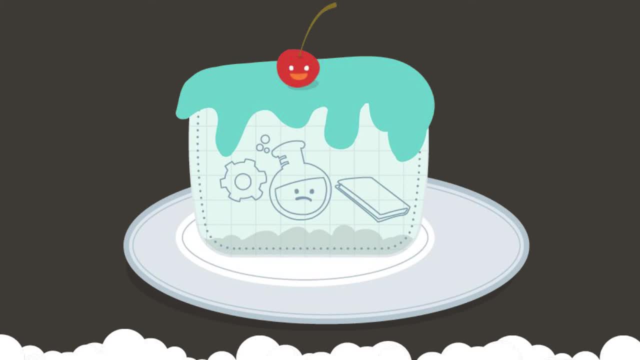 mind in terms of the- you know, the naughty list. the things to not do is that if you ever feel like you've gotten to a spot where your learning objectives are an unfortunate tax or a an unpleasant piece of business, and that you're hoping that your game is some type of- uh candy- 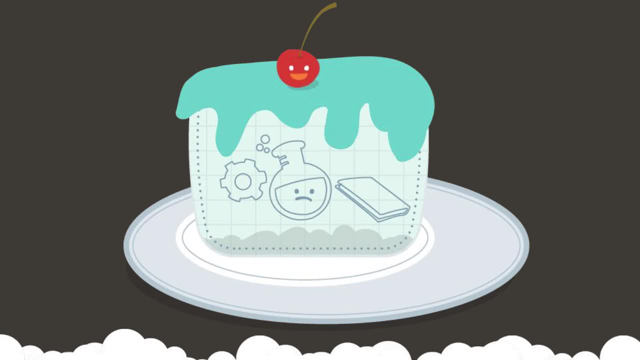 shop Shell or frosting that can conceal what you hope. they know you're. well, you're basically doing it wrong And uh, whenever possible, you should approach your learning objective content as it in itself is an exciting and interesting problem And that knowing it has a purpose. uh, and a. 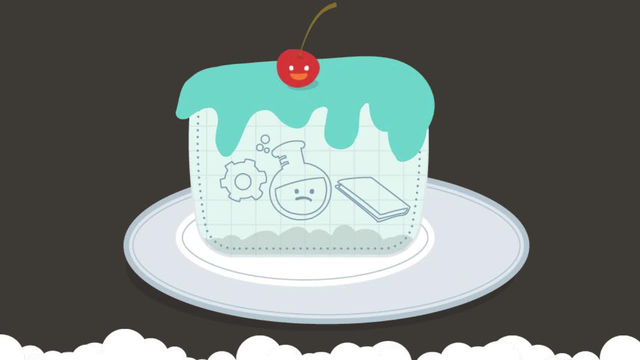 context for it being useful in the learners, Not only just in the side the game experience, but in their life. Um, if you decide that your learning content is in fact, worthless, uh, and that they're, you're using the game as as, as an. 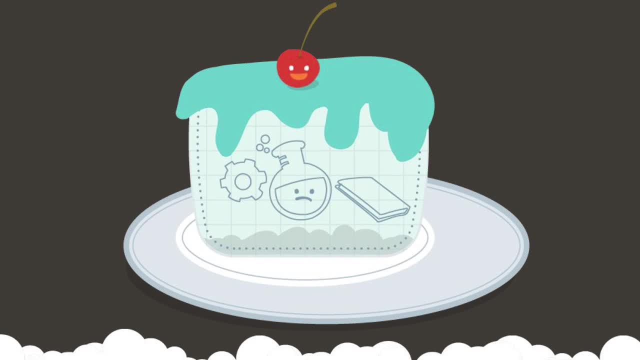 apology or an excuse to deploy that information. you're almost certainly going to make a game that isn't particularly fun And uh and also won't be educational. So you'll kind of fail on both fronts, right You'll? you'll have made a not great game. uh, that is not teaching. 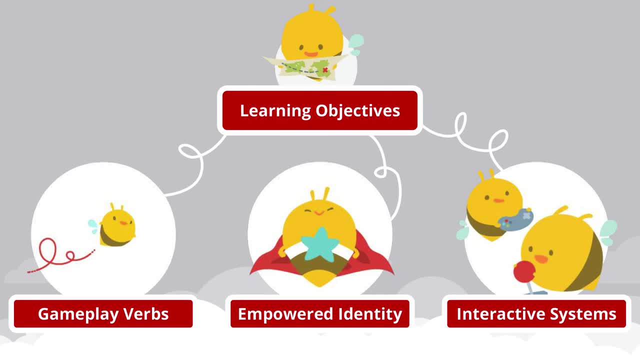 So, to sum up, you should start all of your games with learning objectives that are meaningful and practical. You should have assessments so that you know how to expect what success is on the other side of the project, so that you know what a player will be capable of doing when they've turned the. 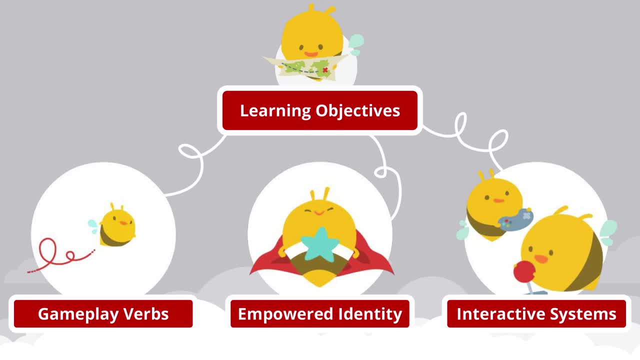 game off And once you have those two things, you can migrate those ideas into the things that a player does, the way the player sees them And the rules that they interact with. If you do all those things, you've probably got a great